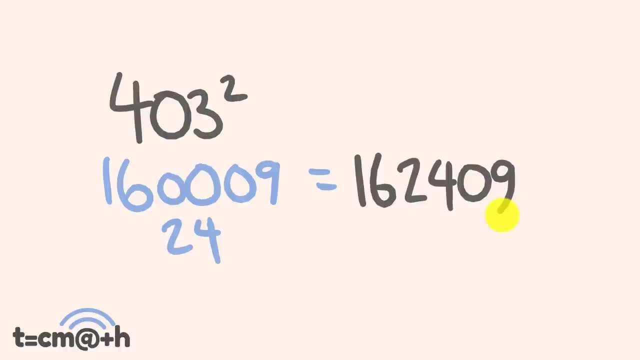 So I'm going to get back to this one and then you can see if you can do it as fast. So I'm going to show you this technique for squaring numbers up to 1000.. But before we get there, okay, I'm going to show you a couple of the smaller numbers first. Just let's walk before we can run, so to speak. Trust me, it's better this way. So, anyway, I am going to come back to this one: 403.. I promise I will, But I'm just going to go through a couple of other ones first, a couple of smaller ones. So I'm going to start with this particular problem here. What about? we do 67 squared? Now, the way that this particular technique works is that we're going to do a couple of smaller ones. 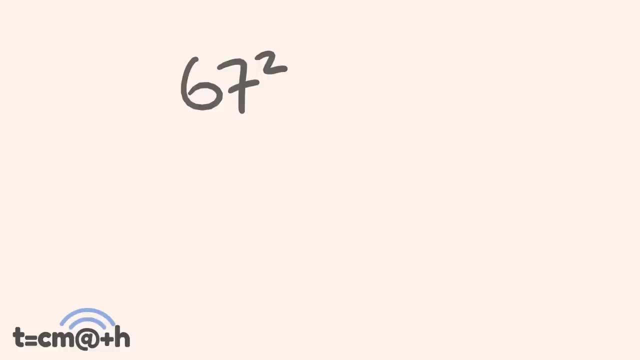 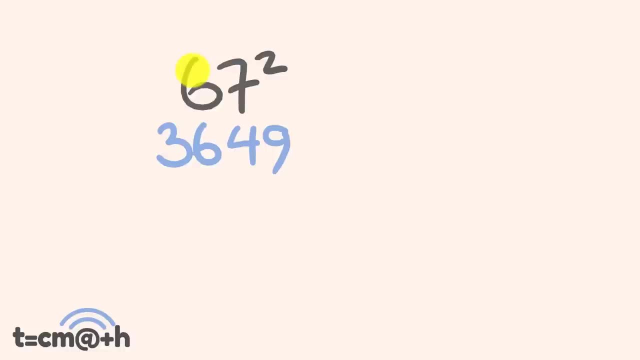 6 times 7, and we're going to multiply then our answer by 2.. So 6 times 7 is a 42. Double that times by 2 is equal to 84.. Now all the same calculations that usually would have occurred. 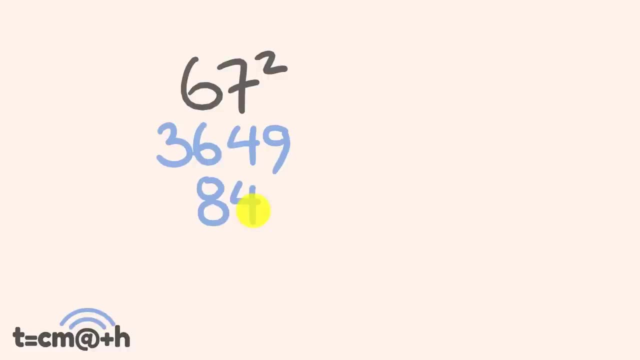 but they've just occurred in a separate order. Now what we're going to do is we're going to add our answer together. So when we do this, we're straight away. what we get is this is a 9.. 4 plus 4 is equal to 8.. 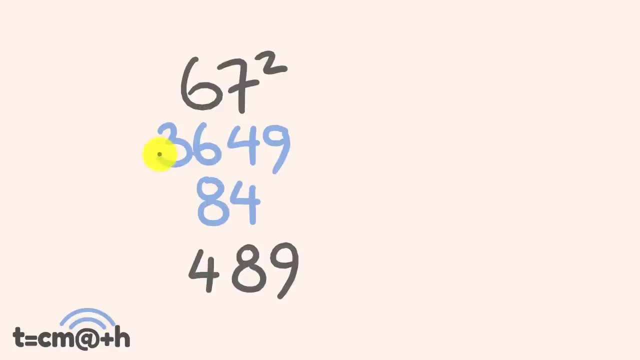 6 plus 8 is equal to 14.. So we carry the 1 there, And 3 plus 1 is equal to 4.. There you go, And that's how this technique works. There is a bit of a tweak for our bigger numbers, so I'll get to those in a second. 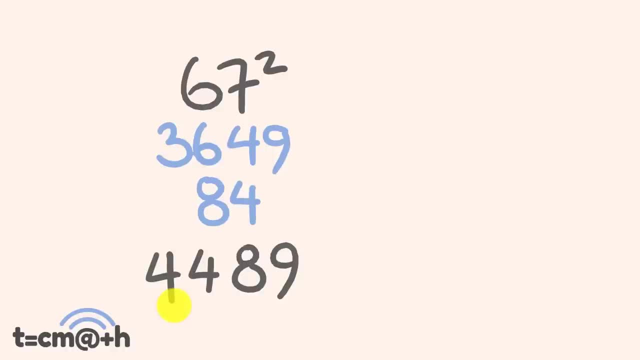 So I'll keep that up there. I'll just go through a bit of a quick recap of what we did, and then I'll give one for you to have a go to, and then we'll get to these big three-digit numbers, right. 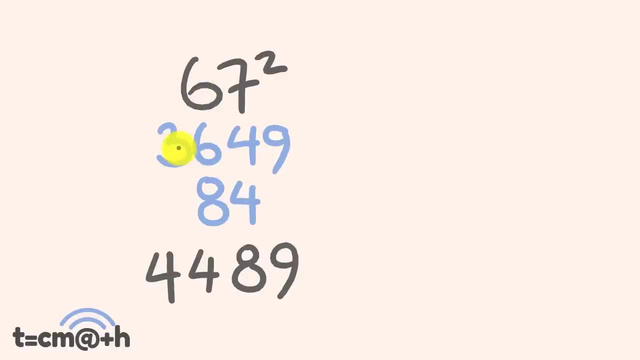 So the first thing is we square this first digit, 6, 6,, so 36.. The second thing, we square the units digit here: 7, 7 to 49.. And then we're going to multiply these two digits and then multiply them by 2.. 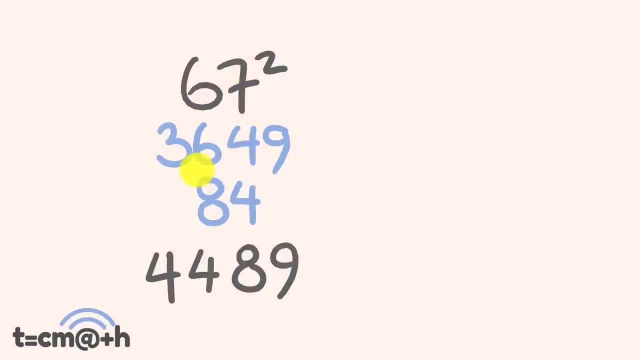 So we've got 84, and then we added the whole lot together. Pretty simple, Okay. so what about I give you one of these? I'm going to keep this one up here, so I guess you can refer back to that. 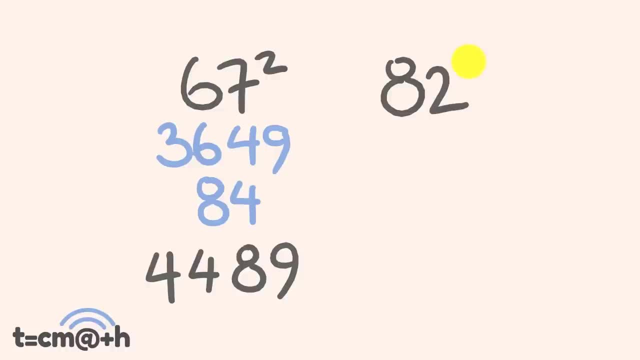 And what about we do? 82 squared. a nice easy one, So give it a go. Now I'm going to go through it. okay, So 8 times 8 is equal to 64.. 2 times 2, we're going to put this down as a two-digit number, a 04.. 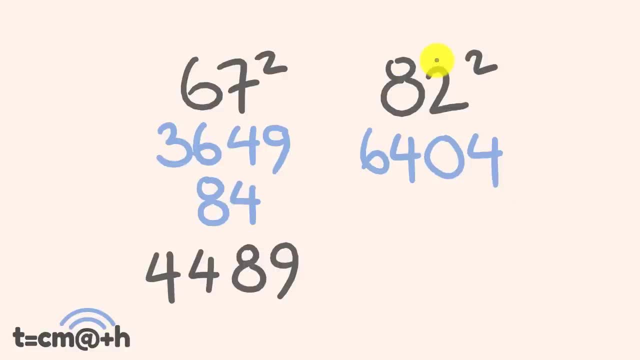 The next one. we multiply these two digits and then we double our result 2 times 8.. 2 times 8 is equal to 16.. We double that, we get 32,. yeah, And now? what do we do? 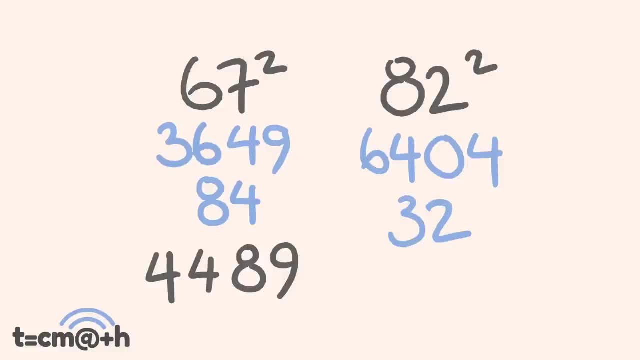 Final step, we add all our answers together And this one we can just add directly over. So 6, 7, 2, 4, 6,724.. So how'd you go with that Pretty? all right, I'll tell you what. now it's the big, ah, the big kahuna burger, I guess. 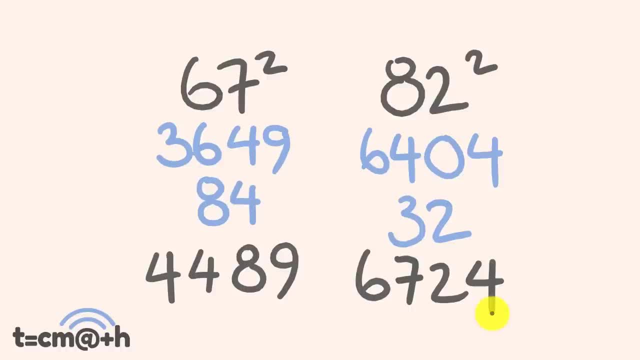 And we are going to get ourselves into three-digit numbers. How to do this with three-digit numbers? okay, The biggest one I guess you could probably pick up from this is if you have something like a four as your answer, or a nine. 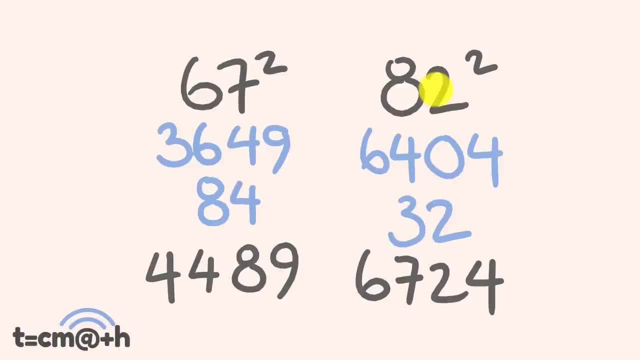 put it down as a 04 or 09, that does matter, okay, So pretty simple, Let's go through and do three-digit numbers. now, The way I'm going to do this is I'm going to go through the first one. 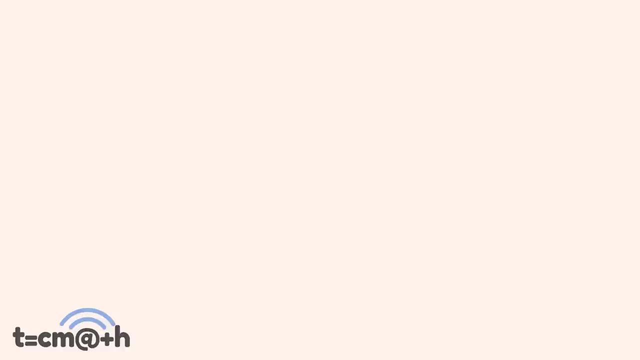 where I'm going to show it to you and how I would approach this. Then I'd give one for you to do and then I'm going to show you that one from the very start there and we'll see how we go with it. 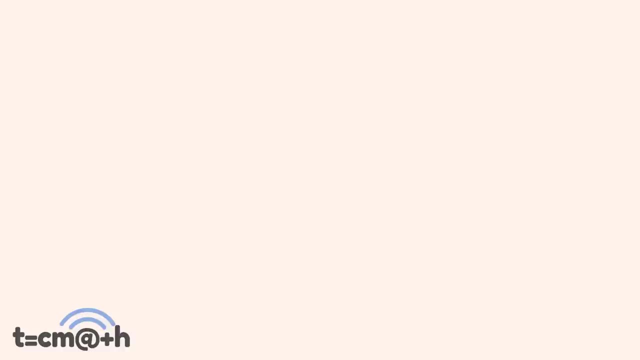 So, anyway, this is much the same as that first part we did, but with a couple of tweaks. So let's just start this out straight away. What about the example of 512 squared? Now, how would I go about doing this? 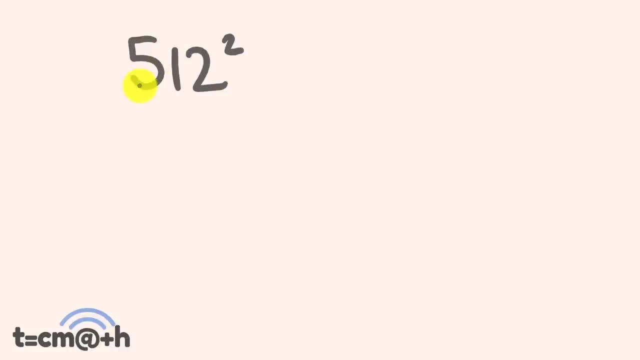 Well, first off, we're just going to go through and square each one of these digits here. So five squared, five times five, is 25.. One times one is equal to one, which we're going to write down as 01,. 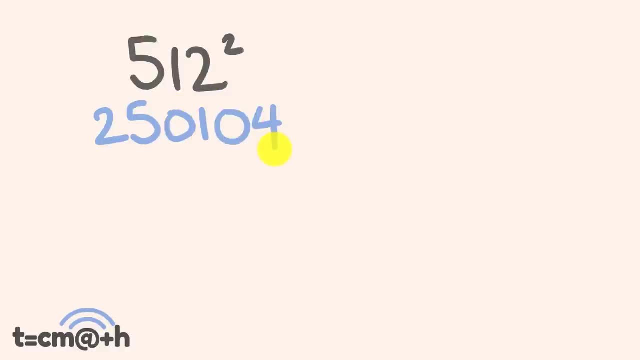 and two times two is equal to four. We're going to write this down as 04.. Next thing, we're going to now multiply these two digits and double it, and then we're going to multiply these two digits and double them and put down our results. 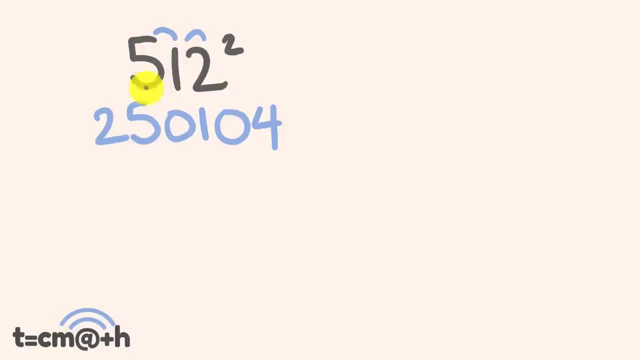 So five times one is equal to five times two is equal to 10.. So I'm going to put that down right here. And two times one is equal to two, And then we're going to double that and we get the answer of four. 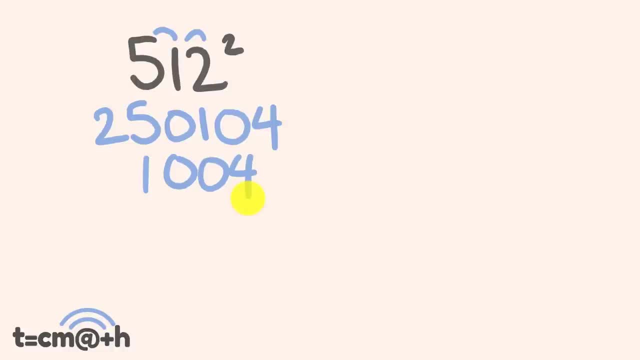 All right, pretty simple. And last of all, we have to do one extra step. We're going to be multiplying the two by the five here, OK, so two times five, And then we're going to double that answer as well. 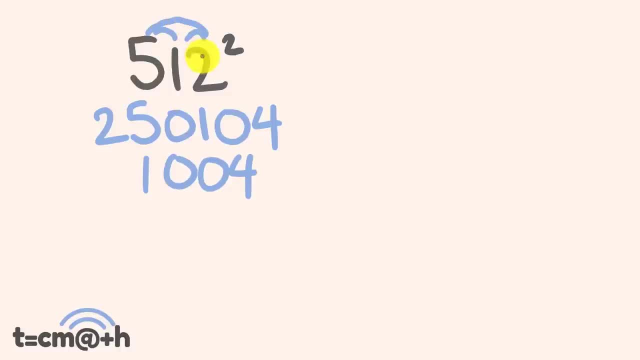 And we're going to dump the answer right in the middle here. So five times two is equal to 10. And then double that. you get the answer of 20.. All right, so now? what do we do? We're going to add all these together. 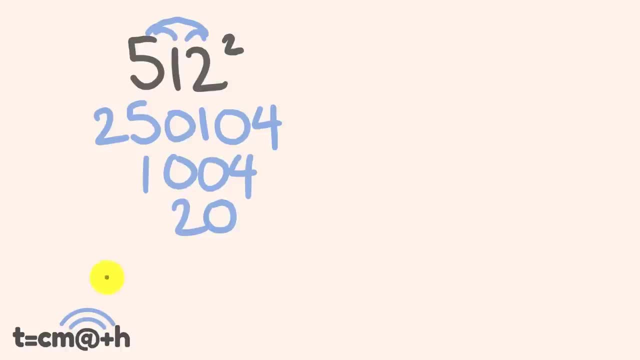 I reckon we can just do these straight down, nice and easy, And let's do that. So this is going to be a two, Five plus one is six. Zero plus zero plus two is equal to two. One plus zero plus zero is equal to one. 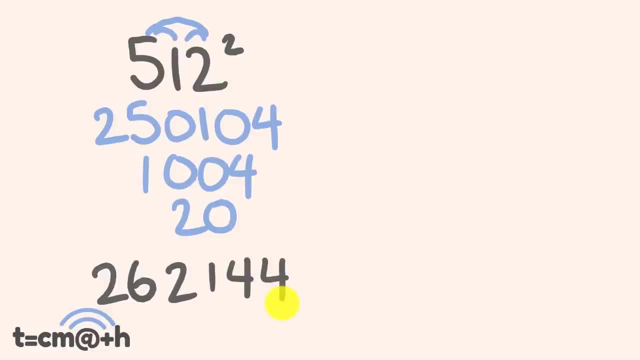 Zero plus four is equal to four, And this one is also going to be a four. Our answer is 262,144.. And, as you'll see, we didn't get away with not doing any of the calculations here. We just did them in a different order. 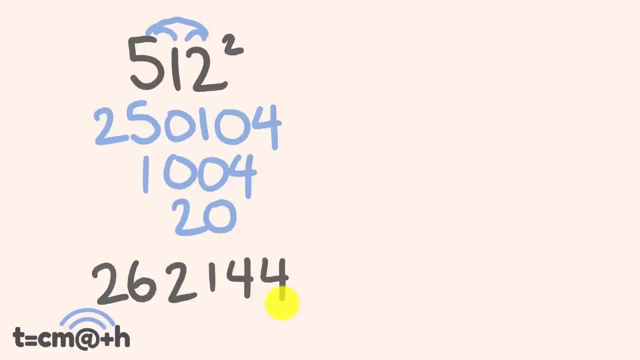 It's just a different technique. Thank you for doing it. You may or may not use it like anything in life. So what about I give you an example to do for yourself right now, And then I'm going to get to that first example which you're going to see. these are really 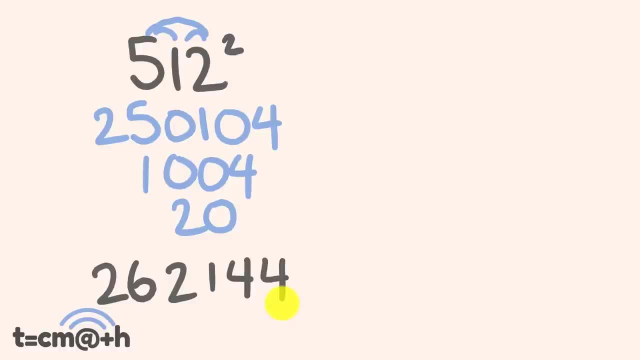 really really quite simple to do. I did choose that one specifically, by the way. So what about I give you one of these? I'm just going to pick a random one here and hopefully get the answer right. What about we do 362?? 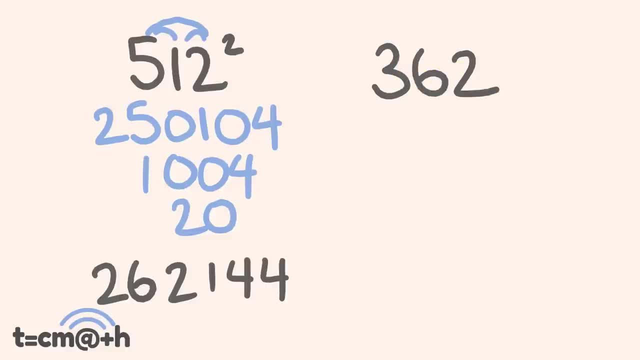 All right, I made this one a bit harder, right? Bigger numbers. I chose a nice, easy one for myself. Choose a harder one for you. Better that you look the fool than me, right? So let's get the first numbers here. 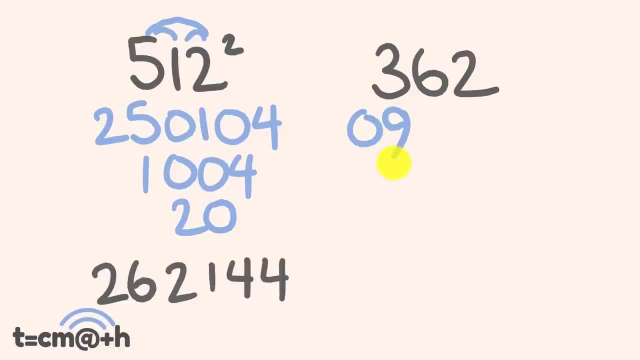 So we square three. We get the answer of nine. I'm going to put down a zero nine. I know we don't need to, but it might help with the placement in a little bit. We're going to square six. next, We're going to get this answer of 36, and then we're going to square two. 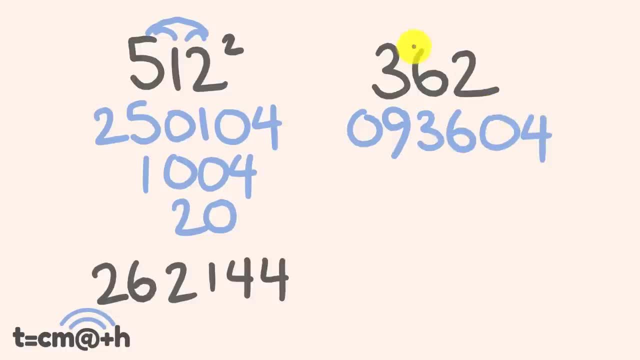 We get the answer of four. Okay, now what do we do? We're going to multiply these numbers and then double them. Three sixes are 18.. Double that, That's going to be 36.. Six twos are 12.. 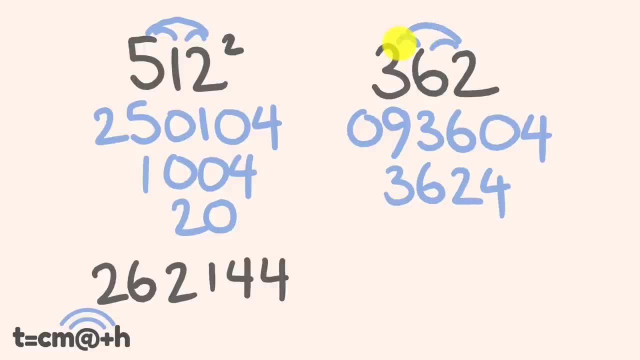 Double that We're going to get 24.. Last of all, Three twos are 12.. Three twos are six. Double that We get the answer of 12.. And we just go through now and add these. I reckon I am going to do this right to left. 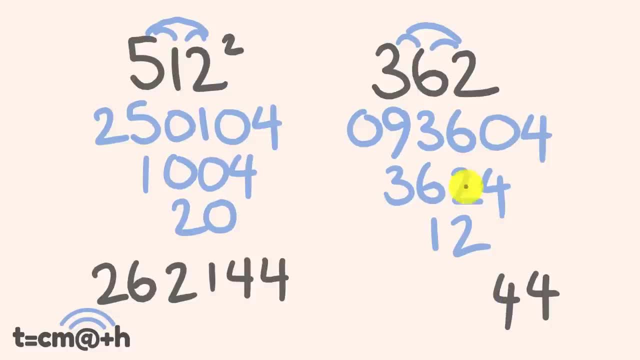 So we're going to get a four here. Zero plus four is equal to four. Six plus two plus two, That's equal to 10.. Carry that one there. Three plus six is equal to nine Plus one is equal to 10.. 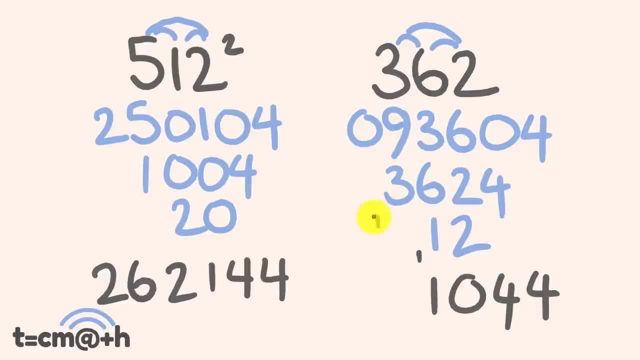 Plus one is equal to 11.. Carry that one And then we're going to get one. plus nine is equal to 10.. Plus three is 13, 131,044.. So how did you go on that? Did you get that answer? 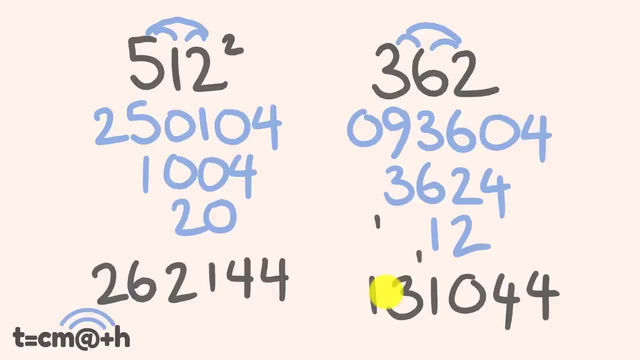 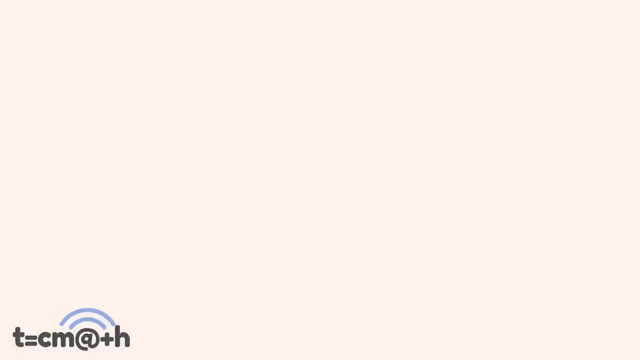 Oh well, It's not a bad technique, right? It's a pretty simple one to do. So now I'm going to show you the example from the very start. Okay, The question from the very start. You thought I would have got to that one first, but hey, going to leave you hanging for something. 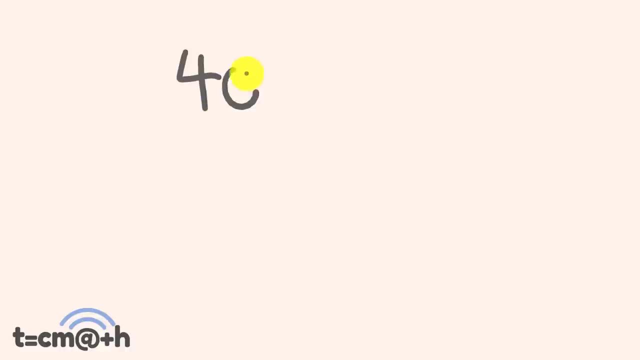 right, And let's put this one down: 403 squared. I reckon you ought to give it a fair fly now and give it a go and see how far she can do it. But I'm going to tell you what makes this easier, because we have multiplication by. 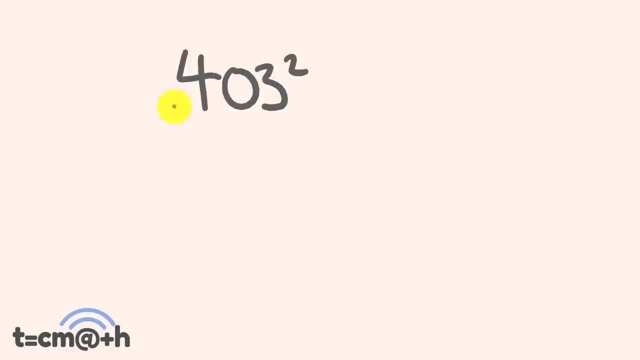 zero. It makes some of these calculations really basic. So four squared is equal to 16.. Zero squared, zero, zero, And then three squared is equal to nine. There you go The next one. we're going to multiply these guys, and then we're going to get zero. 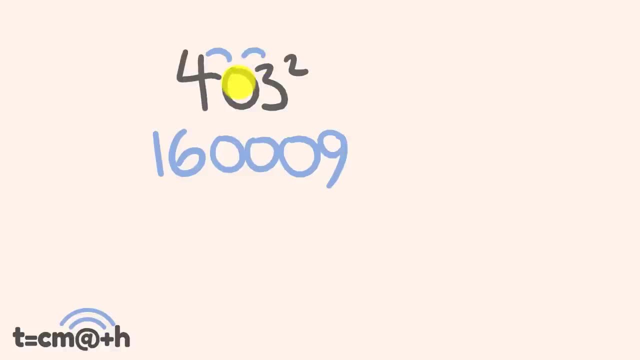 So we don't have to worry about it. We're going to multiply these guys. We get zero, So we don't have to worry about it. The only one we have to worry about is four times three and doubling that, And we're going to dump that right in the middle. 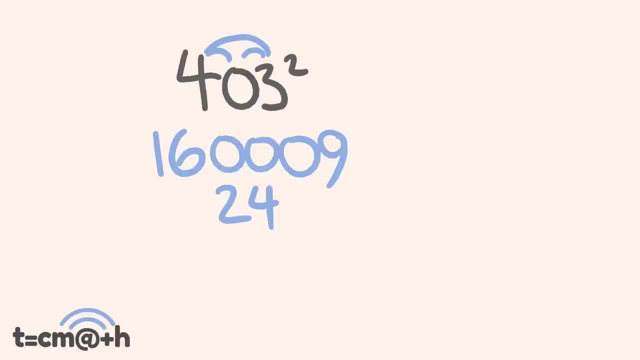 Four, threes are 12.. Put the 24 there And, as you can see, I can just add these straight across: One, six, two, four, zero, nine, And we have our answer right. These ones where they have a zero in the middle, really basic to deal with. 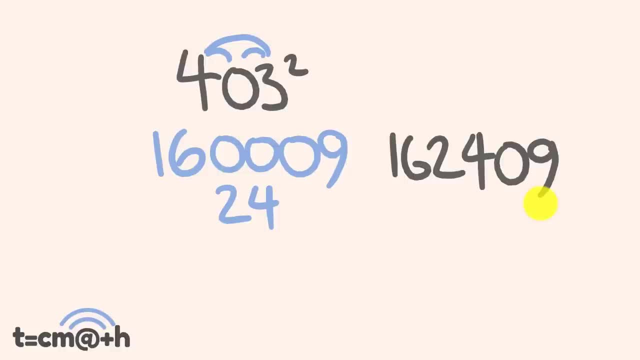 But I'll tell you what. I'm going to give you one of these. Then you can feel really, really smart about yourself. And why not? You've learned something today. You should feel smart about yourself. I'm going to give you one. 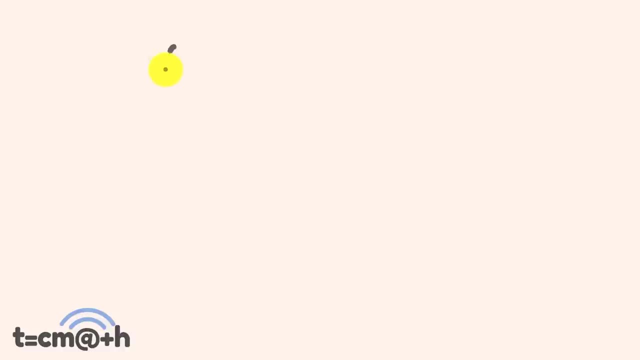 Okay, The one I'm going to give to you: zero in the middle, 607 squared. All right, And see, you should be able to do this pretty quickly. I reckon you can almost do this directly. In fact, I am going to try that, and I haven't tried this before. 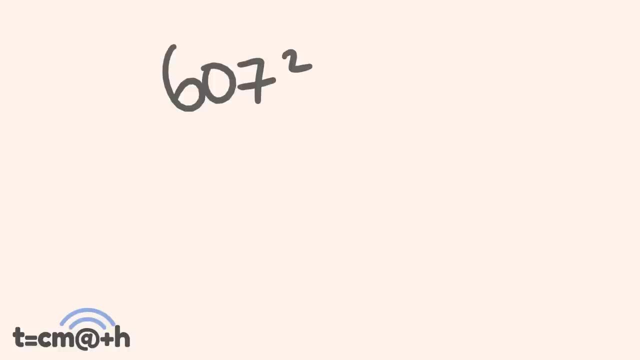 So this is going to be live, So I screw up. Well, I'll probably edit this out, but I don't think I will. So six times six is equal to 36.. Now we know that that zero here is going to put two zeros in the middle. 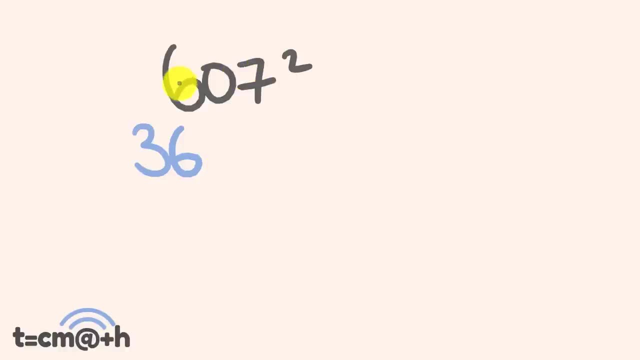 So let's just work at this middle part first, Six sevens of 42 and double that, We're going to get the answer of 84. We know we're going to be adding that on, So let's just do that right now. 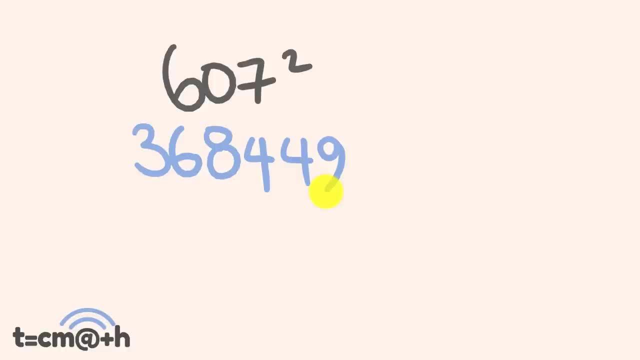 And then seven, sevens of 49.. Hey, pretty crazy, right? We have ourselves our answer straight away. Hey, I reckon that worked. I reckon that was pretty cool. I'm going to give one more of those a go, So let's go. a nice easy one. 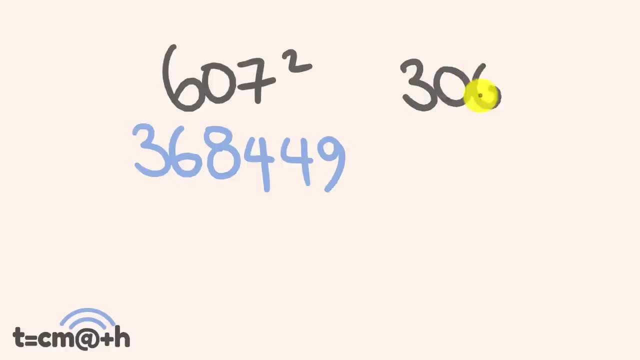 Let's go Three hundred and six squared And I know you kind of look and go. you're choosing easy ones. Hey, they're all pretty easy, right, when you really look at it They're not that bad. So three squared is equal to nine. 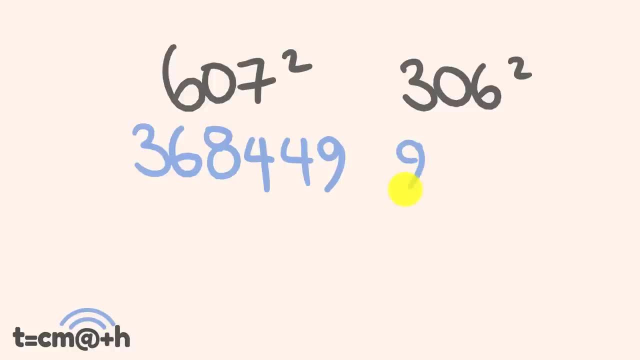 Now I'm not even going to put the zero there, because I know I'm not going to be playing with that later. Zero, zero is going to give me zero, So I'm just going to worry about this part here. Three times six is equal to 18.. 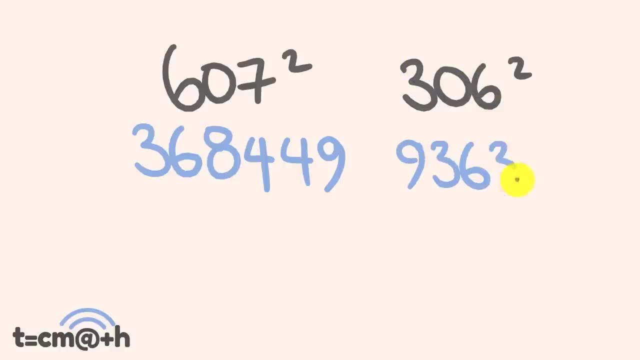 Double that, Going to get the answer of 36.. And then six, sixes 36 is our answer: 93,636.. Anyway, That's a great little technique that I spotted and I thought you might be really interested in knowing. 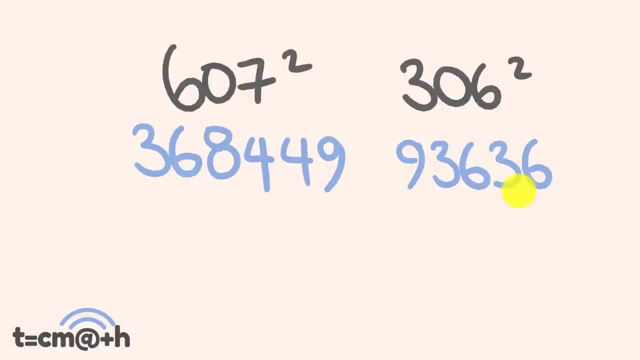 And, if you like it, give me a thumbs up, Put it in the comments. You're going to be probably telling me things like: hey, this is just doing exactly the same calculations, but just in a different order. Hey, I told you that already, right? 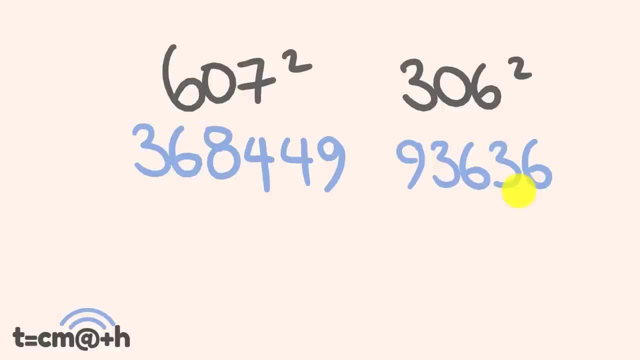 It's exactly what it is Okay With maths. you often can't get away with doing the calculations you have to do. Sometimes it's about working them in a smarter order. So a big shout out to my subscribers and patrons and all you people who have watched and stuck with me this far. 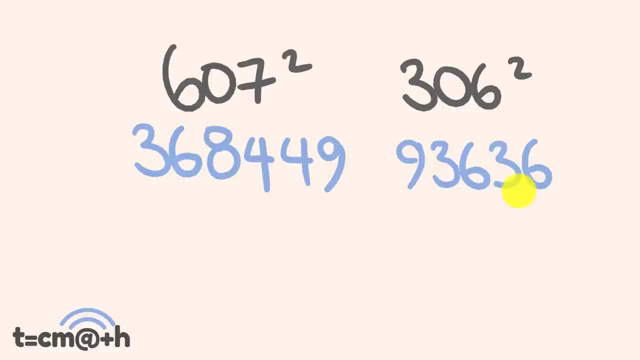 You take care of yourself And we'll see you next time. Bye. 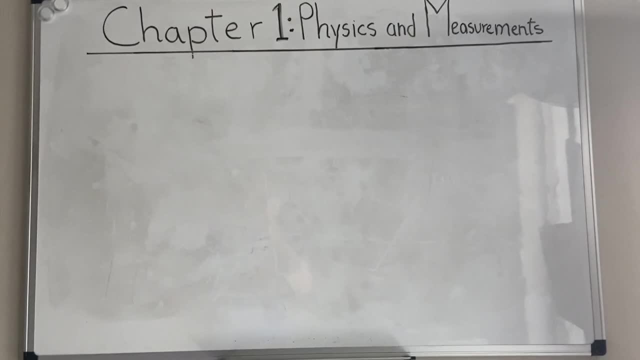 Good morning, guys. I hope you're doing well. Today we're going to go over Physics 1,, Chapter 1, Physics and Measurements. This is going to be a brief rundown of what is said in Chapter 1, and so let's get right into it.